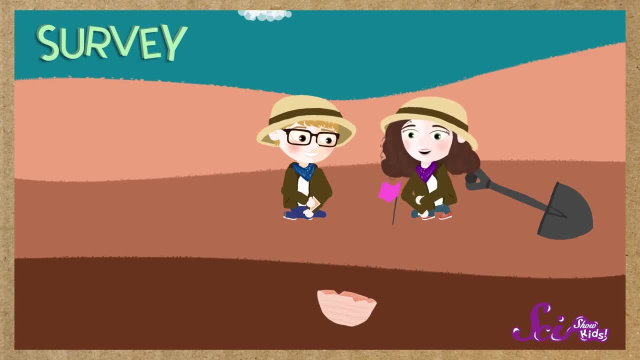 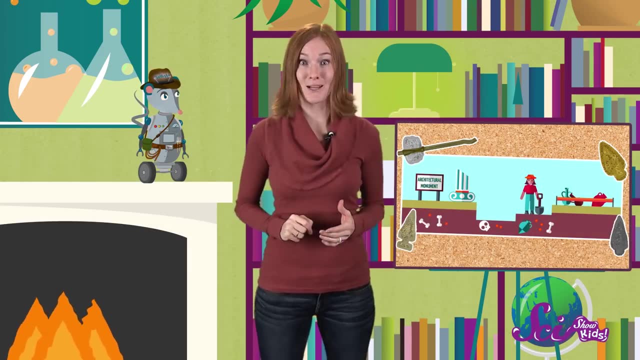 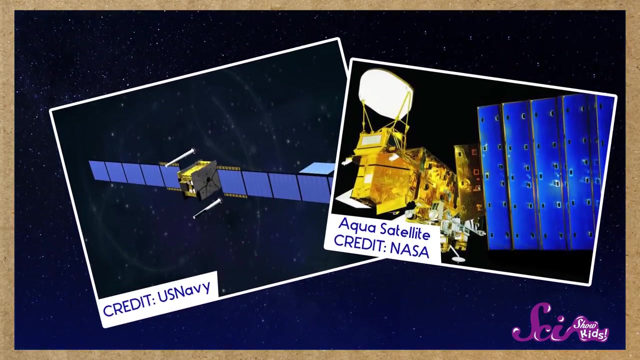 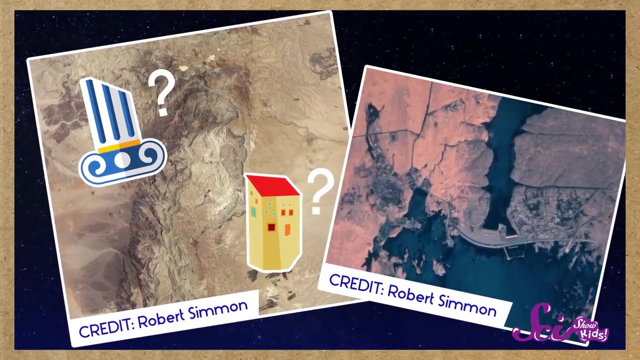 The archaeologists mark these spots with little flags. These are spots where they'll excavate or dig looking for clues, But sometimes archaeologists need to see the bigger picture, So they also survey places by looking at them from the sky. Hundreds of miles up in space. satellites are used by archaeologists to take pictures of places that might have buried buildings or the ruins of other structures that you can't see from the ground. 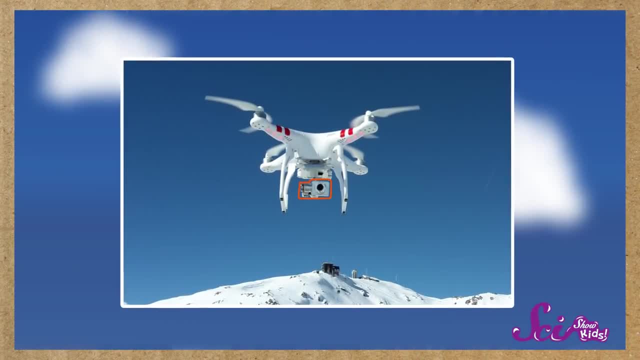 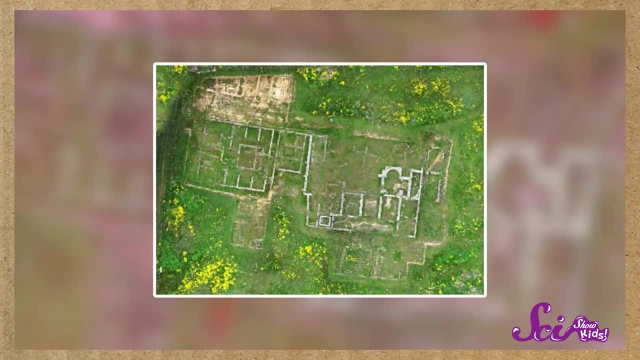 Closer to Earth. some archaeologists use remote-controlled flying machines with cameras on them. By flying up just a few meters or so, these machines can give scientists a bird's eye view of where there used to be something like a house, or maybe a whole village. 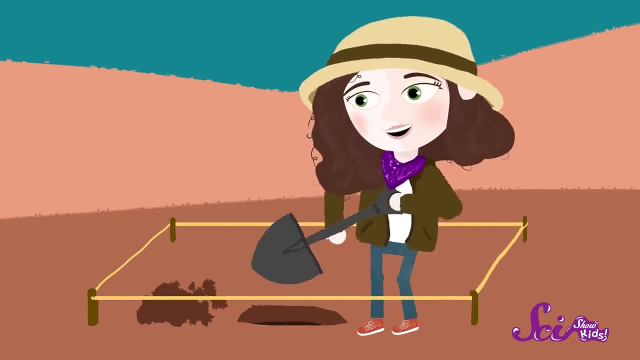 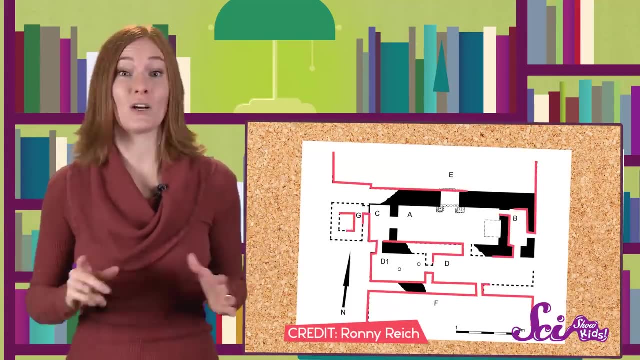 Once archaeologists have found the place they'd like to explore, it's time to get digging. But archaeologists don't just dig in these spots however they want. They carefully map out the whole area they want to explore so they don't damage artifacts in the ground, and so they know exactly where they found them. 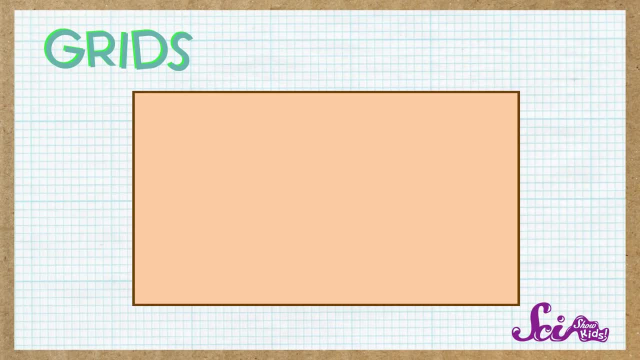 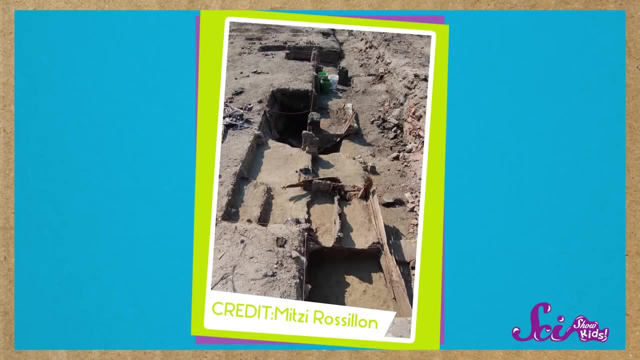 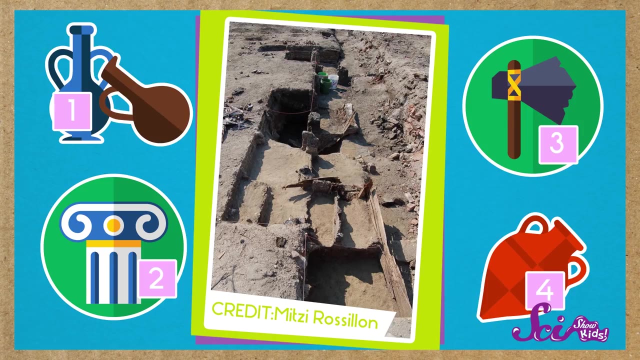 And they do that by using grids. A grid is a design that breaks a section of the ground into small squares. These squares are usually marked with rope and string. Grids help archaeologists keep track of the ground. Each object they find is labeled with a grid number, and then its location is mapped, so archaeologists can remember exactly where each artifact came from. 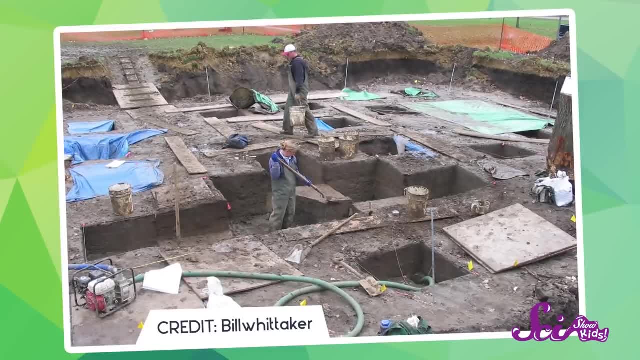 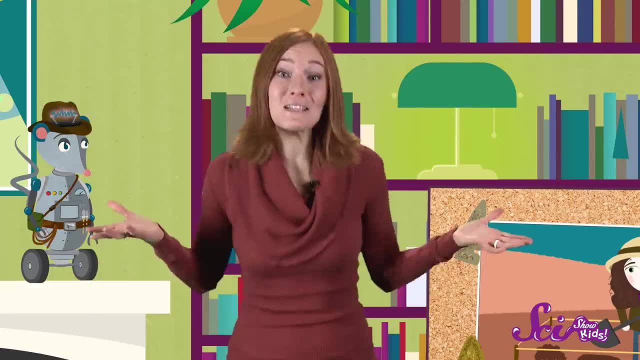 And when they're digging, archaeologists use all sorts of different tools, from spoons and brushes to shovels and even digging machines like bulldozers. So once an archaeologist is done surveying and digging for the day, what's next? 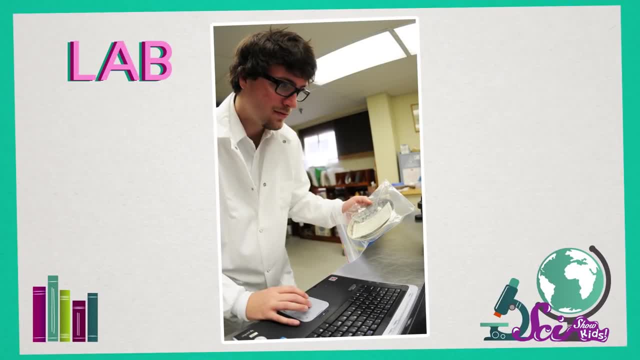 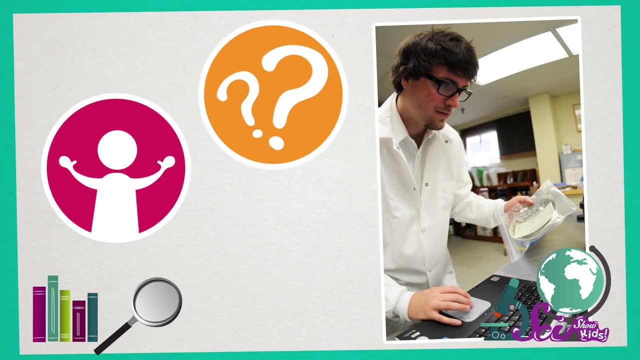 It's time to go to the lab. The lab is where archaeologists get a close-up look at the things they've unearthed There. they start to make guesses about who might have made the artifacts, what they were used for and when in history they might be from. 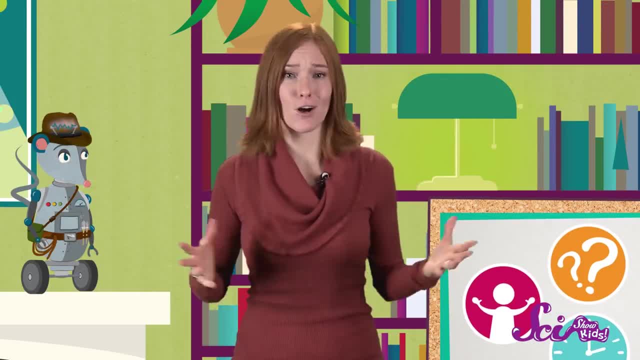 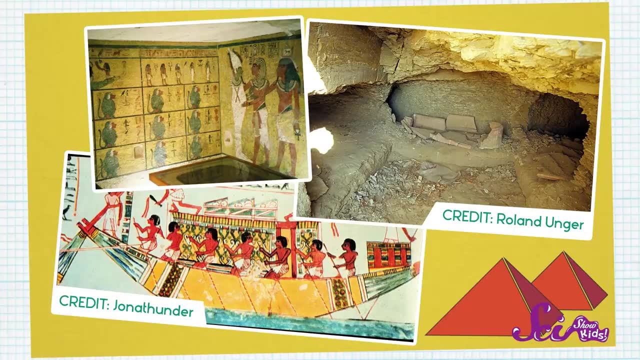 These are the steps that archaeologists use to study how people lived all over the world. Some archaeologists, for example, study ancient Egypt, discovering tombs where people were buried and learning about how the pyramids and other buildings were built thousands of years ago.